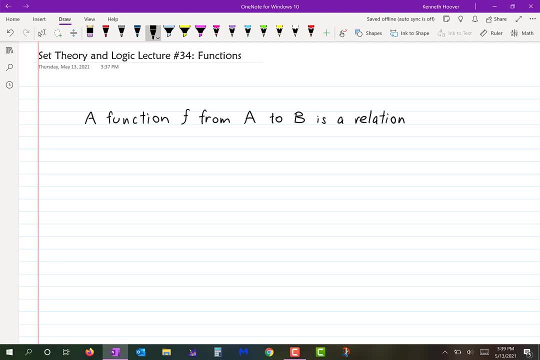 The definition continues. A function f from A to B is a relation A function f from A to B is a relation from A to B, satisfying from A to B. satisfying the property that, the property that For each A in the set A, the relation F. 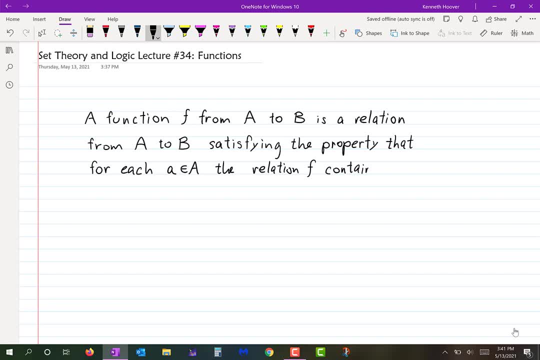 contains exactly one ordered pair. That's the definition. Okay, So let's look at some examples. If I were to draw a picture, let's say: Let's say that this is the set A here, This is the set B. 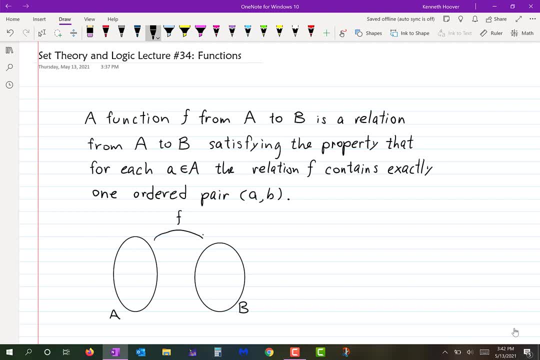 Let's say F is a relation from A to B. Okay, And let's just put some things here. Let's put some things here: Let's say that 2 gets mapped to 0.. 3 gets mapped to negative 1.. 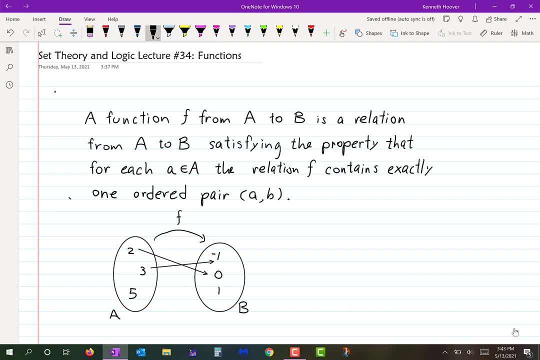 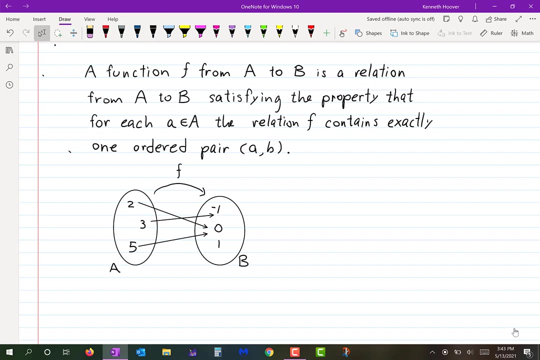 Okay, And 5 gets mapped to 0.. Is that a function? Take a minute and decide if you think that's a function. Okay, The answer is yes, Let's draw this function, Not draw, Let's write the function out. 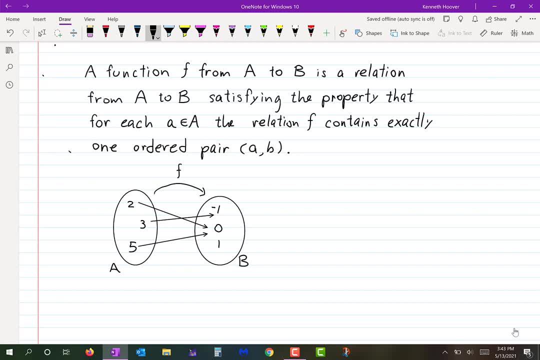 What is a function actually? What's a relation actually? We talked about this last time. It is actually a subset of A cross B, Right? So this relation here is literally the set of ordered pairs, And there's 3 of them. 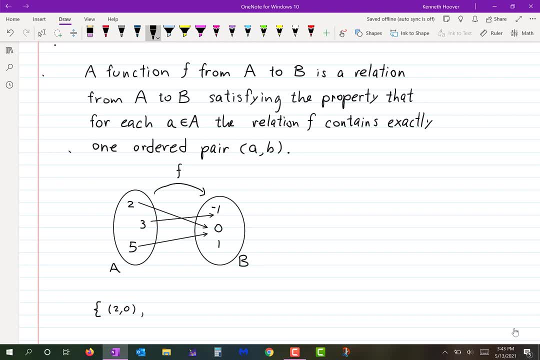 There's 2, 0.. There's 3, negative 1. And there is 5, 0.. Do you see that for each element of A there's exactly one ordered pair starting with that element Right? The elements of A are 2,, 3, and 5.. 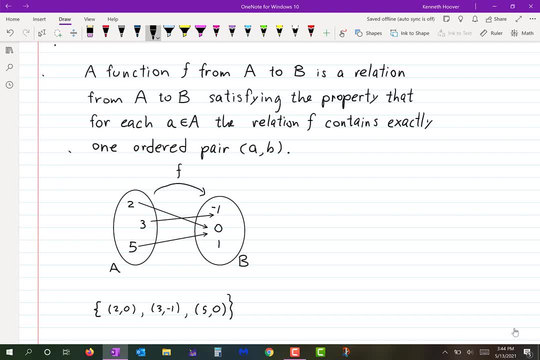 There's exactly one ordered pair starting with 2.. There's exactly one ordered pair starting with 3.. And there's exactly one ordered pair starting with 5.. So that is a relation. Now, if I added in here an arrow, 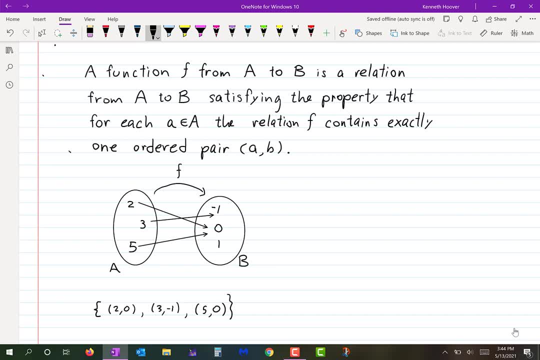 I'm sorry, That's a function. It is a relation, of course, no matter what, But it is also a function. Okay Now, if I added in here another arrow, Let's say that we send 3 not only to negative 1, but also to positive 1.. 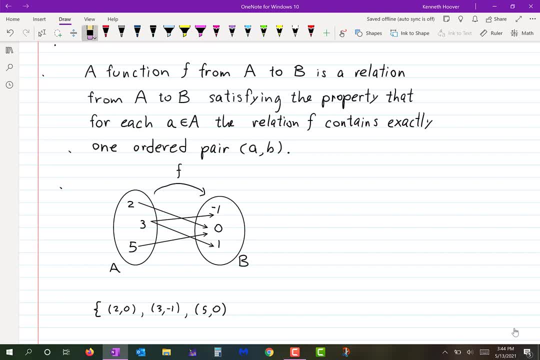 Then it would not be a function, Because there would be 2 ordered pairs, starting with the number 3.. Okay, Alright, So let's put that back to where it was, so that it is a function. There we go. Notice that 1 is an element of B, but it is not being used by this function. 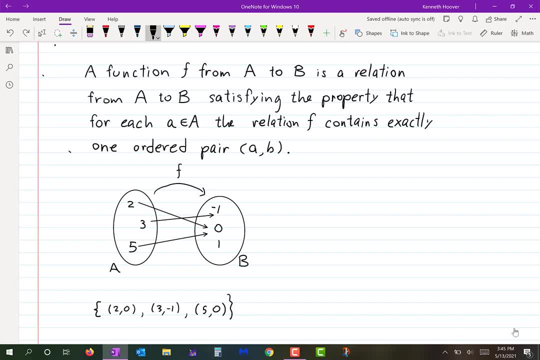 That's why B is not called the range. It's called the codomain. The range is just the set consisting of negative 1 and 0. The range is a subset of the codomain. It might equal the entire codomain, but not necessarily. 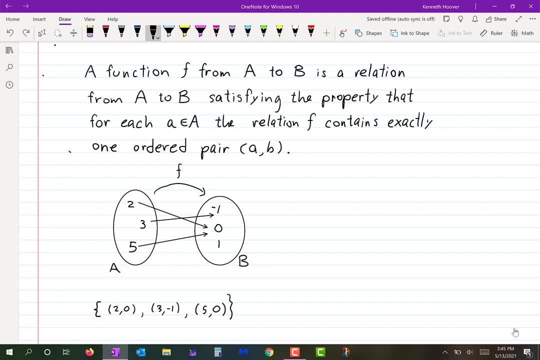 Okay, Now, When you have a relation that happens to be a function, then we allow ourselves to write, for instance here, let me write this down: If AB, the ordered pair AB, is an element of F, that's actually correct to write that. 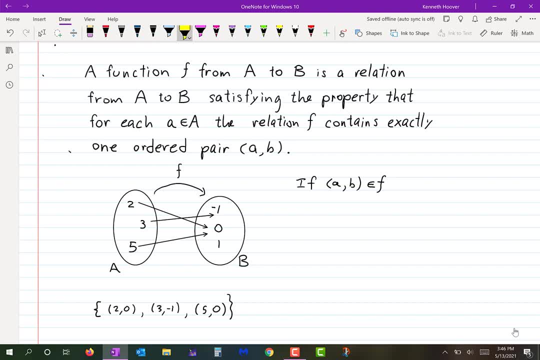 to say it's an element of F, Because this is F right here. That set of ordered pairs is the function F. A function is in fact a set of ordered pairs. Okay, So it is correct to say if AB is an element of F, but I haven't finished the sentence. 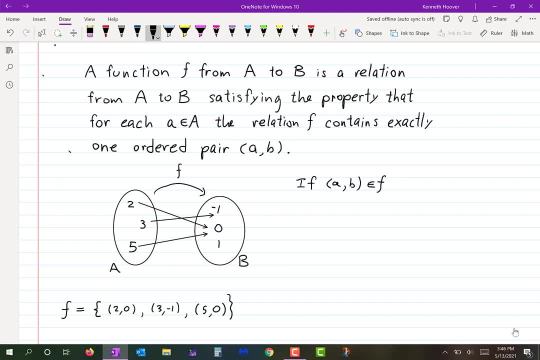 That's the hypothesis of a conditional statement. Where's the conclusion? Then We write: F of A equals B. You do not write that unless the relation F is a function. If F was not a function, a non-function relation, then you would not write F of A equals B. 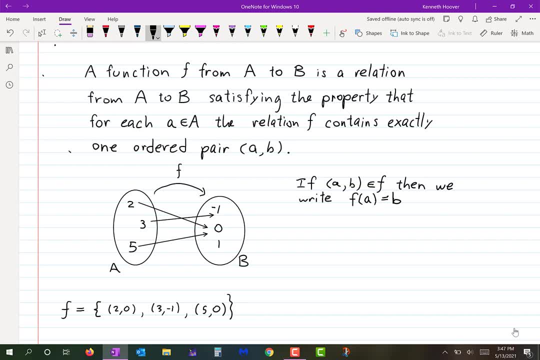 Okay, Here's something else too. Is that you're used to seeing this? I know you are. You're used to seeing this: F, colon A, arrow B, That's how we write. F is a function from A to B. 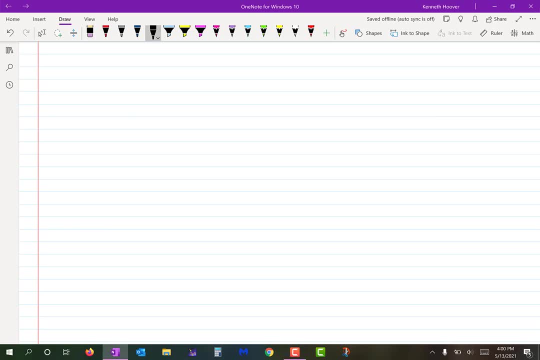 Okay, Now suppose we have a function F from A to B. I'm going to give some definitions now. Okay, It's a defined function, but I'm going to give some other definitions. Okay, So, first of all, here is just what I would call. I mean, I guess these are definitions. 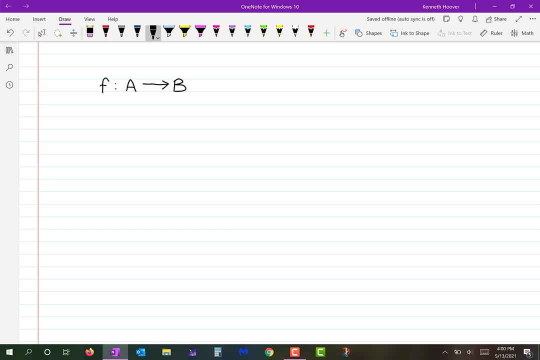 but I just call them statement of fact. Okay, A is called the domain of F, B is called the codomain of F. You already know that. That's another reason why I'm not really referring to these as definitions, because these are. 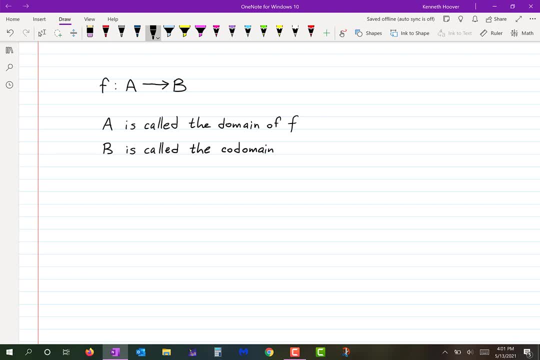 terms that we've been using already for a whole lecture and a half. so far, Okay, But here's some new stuff. I'm going to be more specific right now about what the word range means. Okay, Okay, I'm going to write it like this: 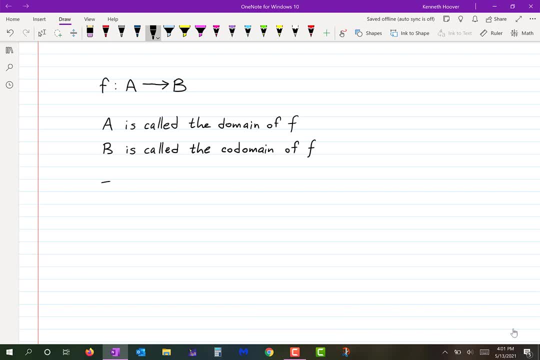 The range of F is the set of all elements of the codomain. Okay, I'm going to write it like this: The range of F is the set of all elements of the codomain. Okay, Such that there is an ordered pair in F containing B as the second coordinate. 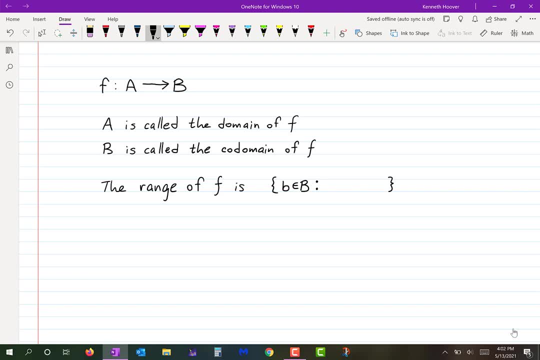 So, in other words, I'm going to say the set of all B in the set B, such that there exists an A in the set A. I need some more room, Such that AB is an element of F, Okay, Or an alternate definition. 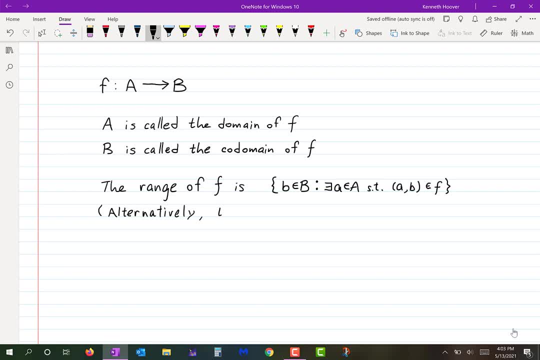 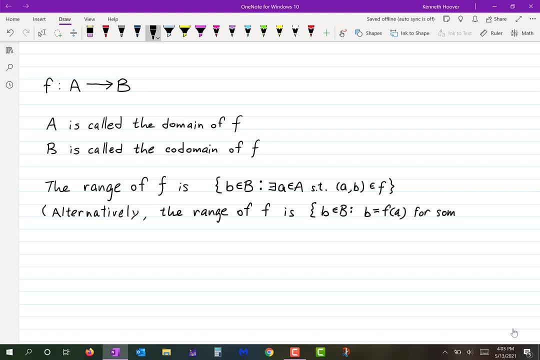 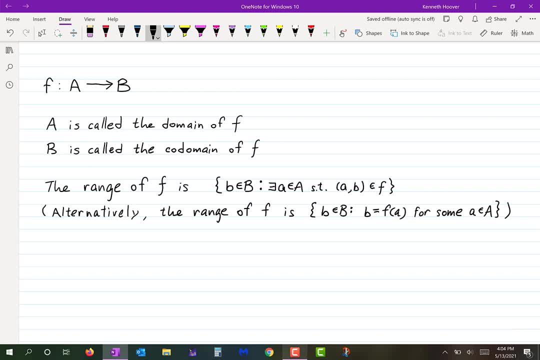 okay, F is surjective, or another way of saying that is a surjection, if, for all be in the codomain, there exists some a in the domain such that be equals f of a. ok, that's a surjective action. another word in place of surjective, this a minute here. 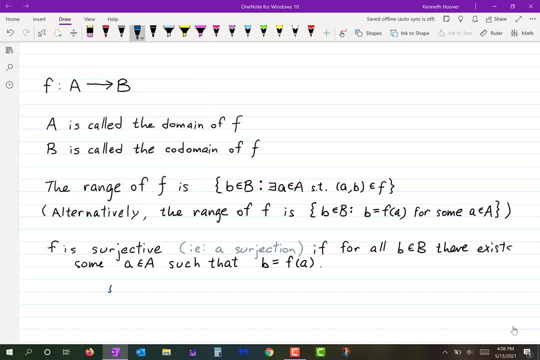 ok surjective is oftentimes also called any trouble with my pen, again today because of the heat. ok surjective is oftentimes also called onto. you would say it doesn't make sense really to say F is onto that. that's not really proper grammatically. but what you would do is 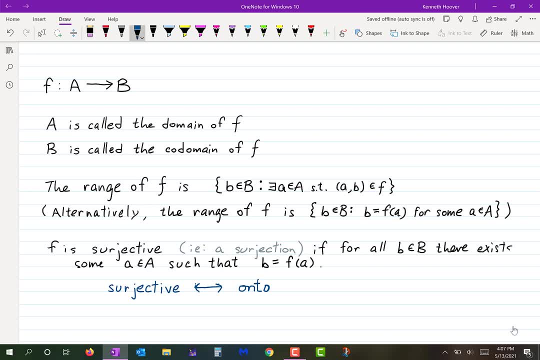 you would say F, maps a on, to be ok. and also I want to point out something: what does that mean? if you look at that definition, isn't that definition just saying that the range is beat? that's all it's saying. read it again, if you didn't. 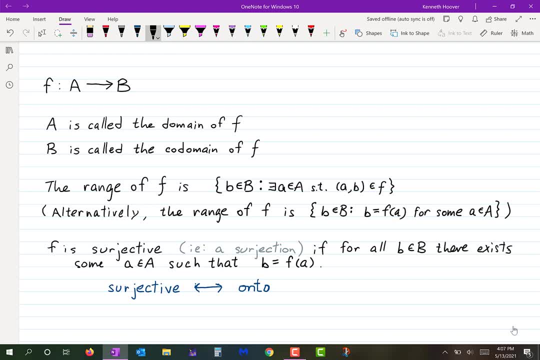 notice that. then read it again and notice that emphasis: objection if the range is the whole codomain. ok. now I want to point something out to you that a function here. this is important. all three of these things are really part of the function, the function itself, what we call the. 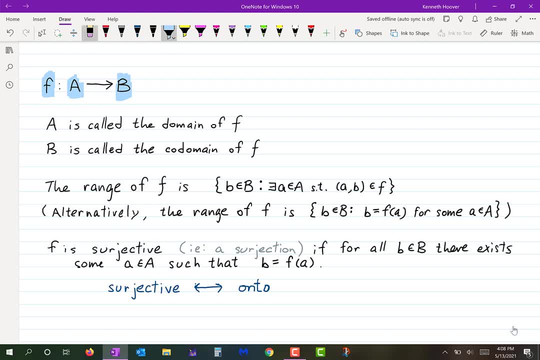 function, but also the domain and the range are part of it in some sense, and what I mean by that is this: let's think of the square root function. ok, let's think of the square root function. what's the domain of the square root function? it's all non-negative numbers. 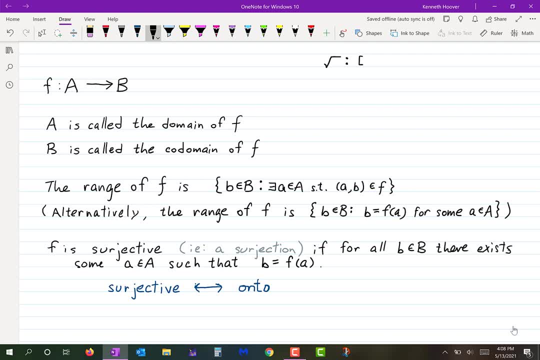 right. so I didn't mean to put a one there, I meant to put infinity, that's the domain of the square root function, right? so the third function I'm going to put is a. All right, What's the codomain? I'm not asking for the range, I'm saying the codomain. Well, here I'll tell you this. There's actually billions of different answers. You can all give a different answer and I'll be correct. 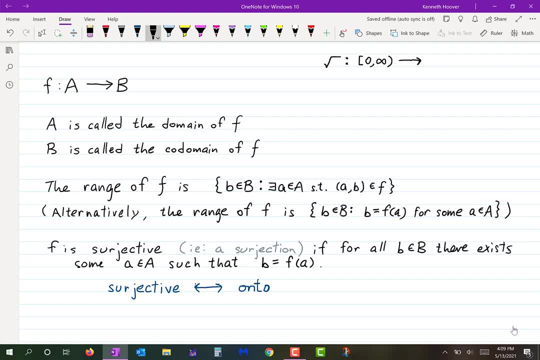 All right, I'm going to be the most general and say that the codomain is the real numbers. That's true, isn't it? Isn't it true that the output of the square root function is always real? Right, When you're plugging in a non-negative number into the square root function, you get a real number as an answer. 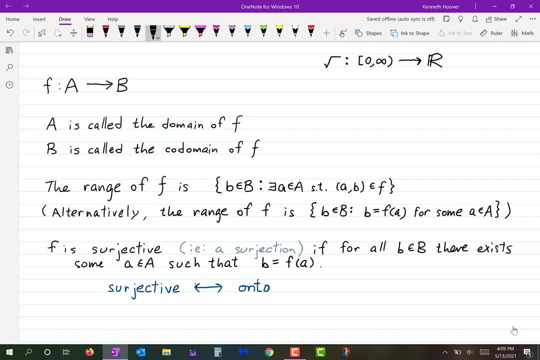 If I here just for the sake of argument, let me tell you this: We're not going to do this in this class, but I could have done this and that would actually be correct, wouldn't it? if I put the codomain as the complex numbers. 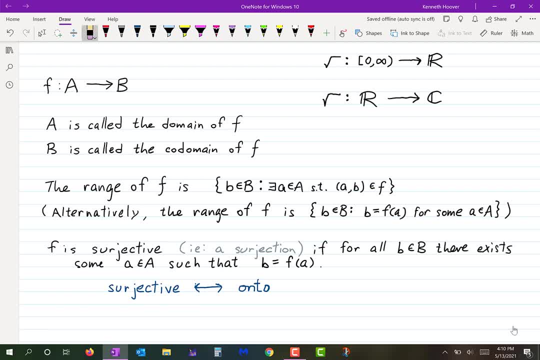 That would be correct too, But that's not what I want to do right now. Let's just think about real square roots. okay, So what I have written there is accurate, is it not? Yes, it is. Is that written there? is that a surjection? No, it is not, because the range of the square root function would not be all real numbers. 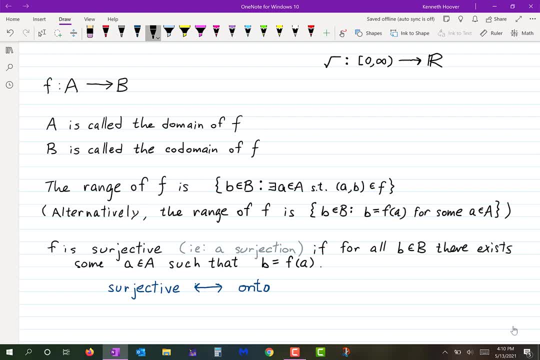 When you plug in a non-negative number into the square root function, you only get a non-negative real number. So that is not a surjection. Now, this is also correct. That is also correct, is it not? That second function is a surjection. 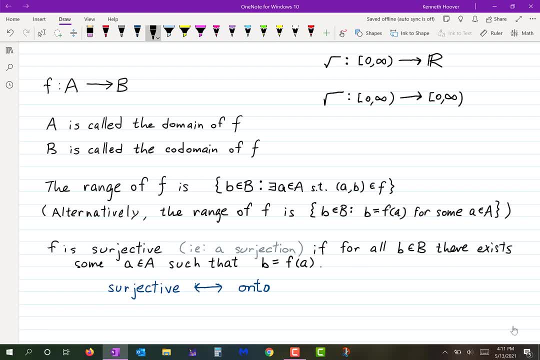 So it's the same function though, isn't it? So what that tells you is that, philosophically, when you say I have a function here, what you put as the domain and the codomain are actually the same. So it's actually kind of part of the function in a way here, because in one philosophical sense these two functions are the same function. 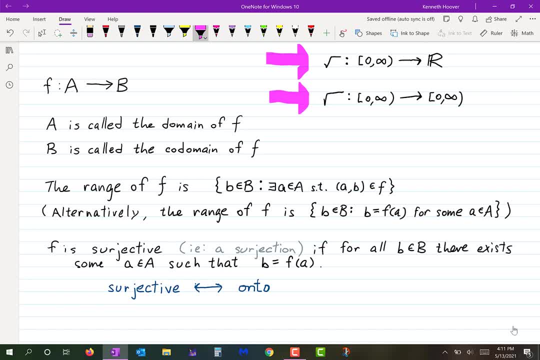 But in another philosophical sense they're different because the second one is a surjection and the first one isn't, So there's some intricacies that you have to be slightly careful with. Okay, Definitely, I would say this: There's usually no confusion. 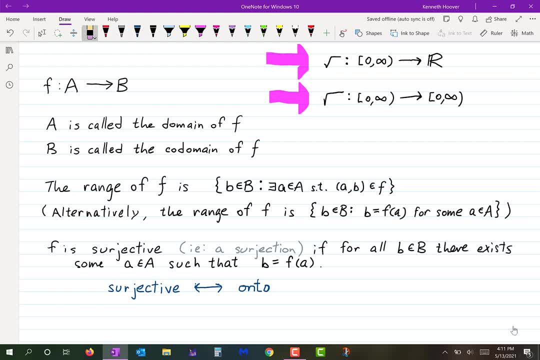 Okay, Definitely, I would say this. There's usually no confusion. Okay, Definitely, I would say this. Definitely, I would say this: You can avoid confusion by just paying attention to the context. But definitely this: If the word surjection or surjective or onto is being thrown about. 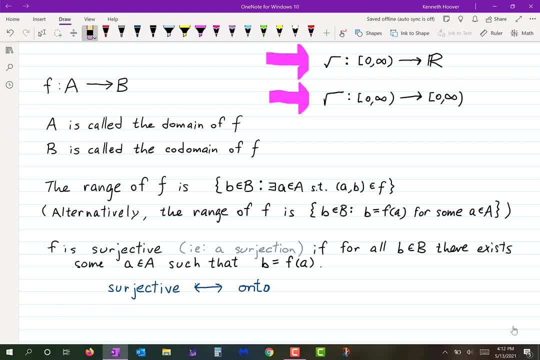 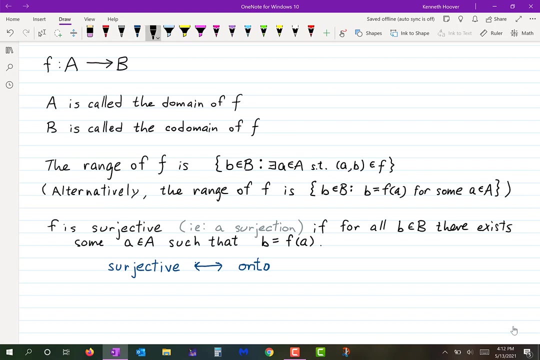 then it's very important what is being written down as the codomain, because, in order to use the word surjection, the codomain can't be any bigger than the range. Okay, Let's move on. There's another word, which is injection, or injective is the adjective. 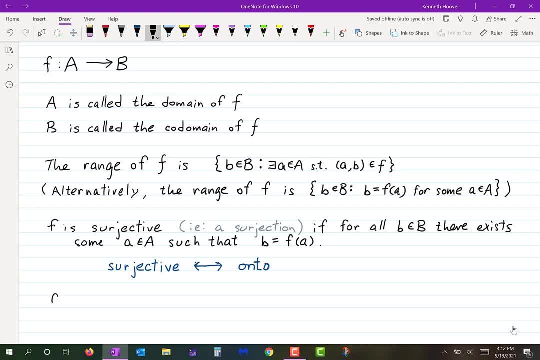 Injection is the noun Okay, F is injective, In other words an injection, Injection, Injection, If For all A and A prime in the set A. Now let me stop and describe that prime for a second. That A prime doesn't mean that you're doing something to A. 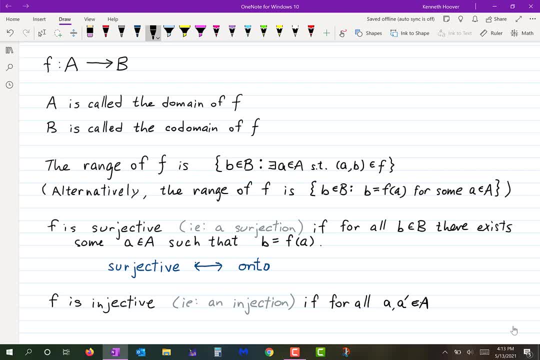 It just means there's two different elements of a and they didn't want to say a and b, because for this whole lecture we've been using b to stand for elements of set b. okay, so they wanted they wanted to say here two elements of the set a. so 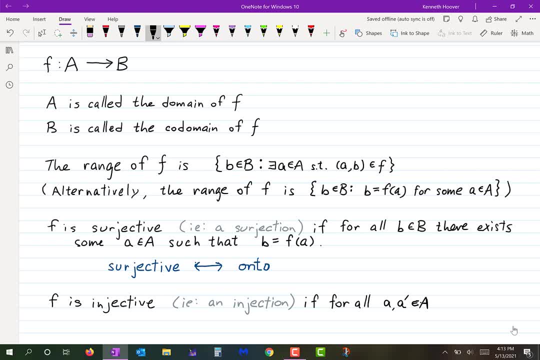 you call one of them a. that's pretty obvious- and then the other one you call a, with some extra decoration on it to differentiate it from the first element that they said and and uh, sometimes people will put a with a tilde over it, some people put a with a hat over it. this book just happened. 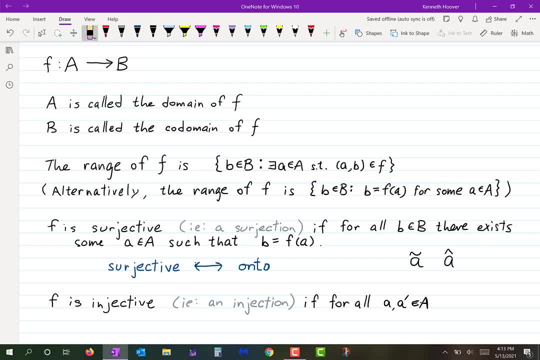 to put a with a prime on it. okay, all right, let's get back to the definition. f is injective if, for all a and a prime in the set, a, with a not equal to a prime, we have. f of a does not equal f of a prime. 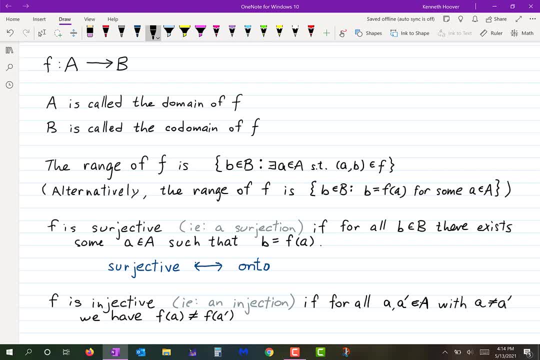 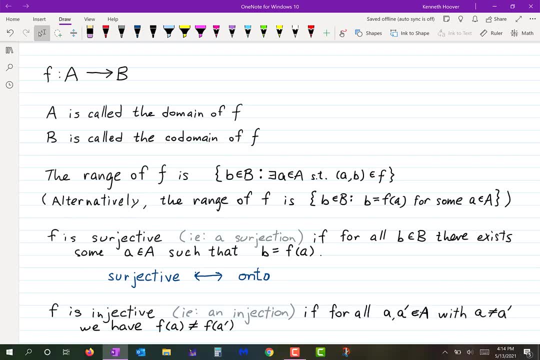 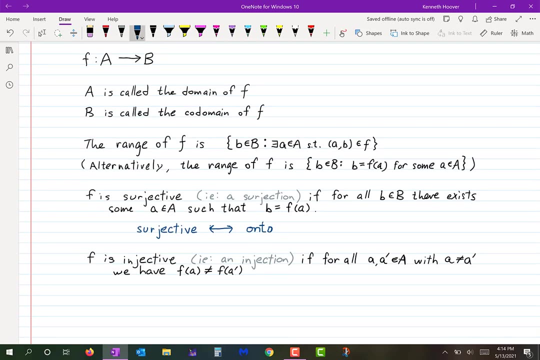 okay. now there's a very common other way of saying in injective that you should become familiar with if you're not already: okay people. oftentimes, instead of using the word injective, they will oftentimes say one to one okay and one more f is bijective. 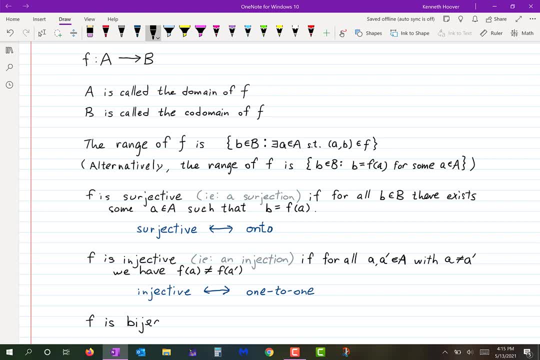 in other words, a bijection if it is a bijection, if it is a bijection, both injective and surjective, and what would be the other way of saying that one to one and onto? okay, now here's some things that i like to use. these aren't really official symbols, but 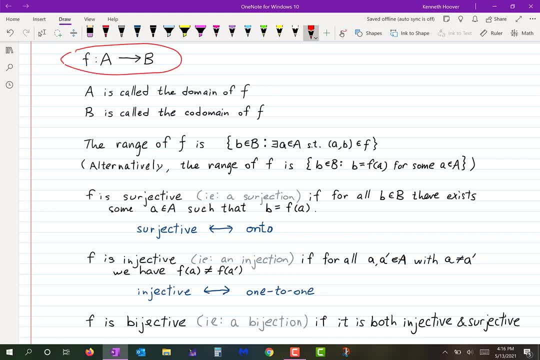 i like to indicate, when i'm writing something like that, when i'm writing f as a function from a to b. i like to have a way to indicate there if it's an injection or a surjection or both, what i do. i don't always do this, but but when i want to. 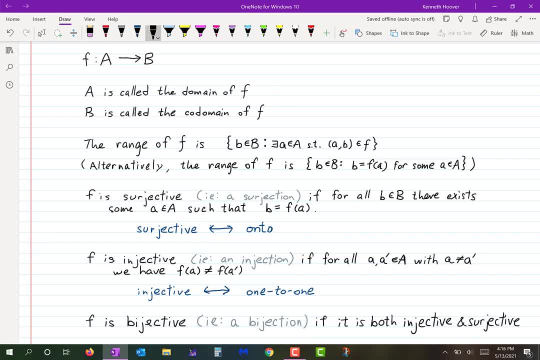 indicate that. here's how i do it: if it's an injection, then i write 1-1 above the arrow, and if it's a surjection, then i write onto 2 below the arrow. not every mathematician does that, but i'm not the only one. 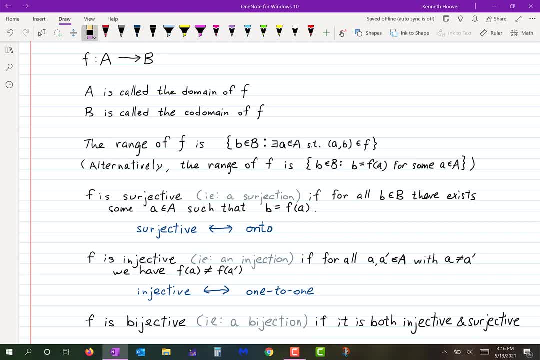 but i do think it's nice to have some way of indicating injectivity and surjectivity. okay, now i would like to do a couple things. i would like to just walk through with you an outline of how would you prove a relation is a function, how would you prove if it's injective and how would you prove if it's surjective. okay, 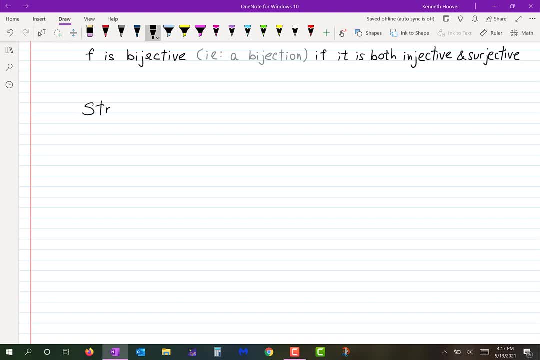 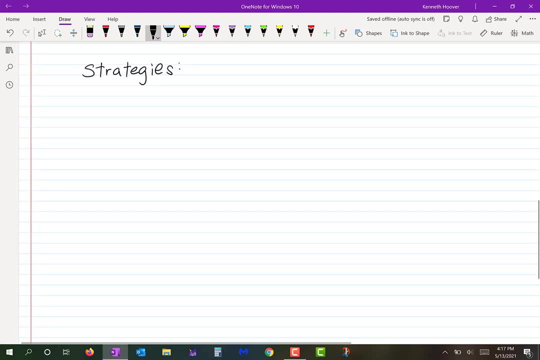 so these are strategies for proving these types of things. okay, so, given a relation f f from a to b, or we can say into b- i can't say onto b because i don't know yet. okay, given a relation from a to b. okay, we can prove. 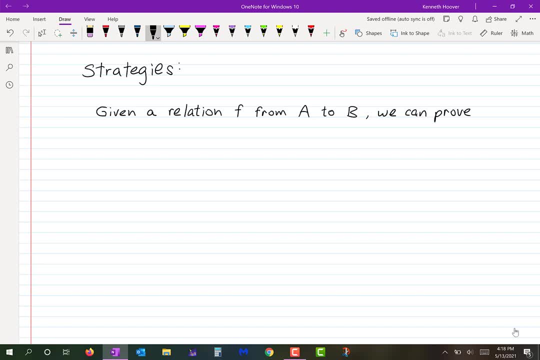 f is a function, only if it really is a function. I mean, you can't prove it's a function if it's not. So I'm saying: you know what? if they say: here's a relation, prove that it is a function. 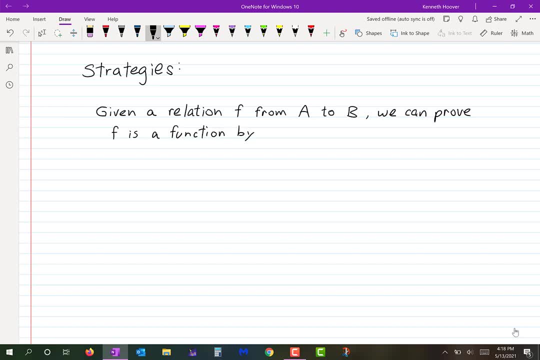 How would you do that? Okay, so we can do that by okay, One way is to say: well, I say one way, but this is really the way to do it, the standard way to do it. okay, What you do is you suppose? 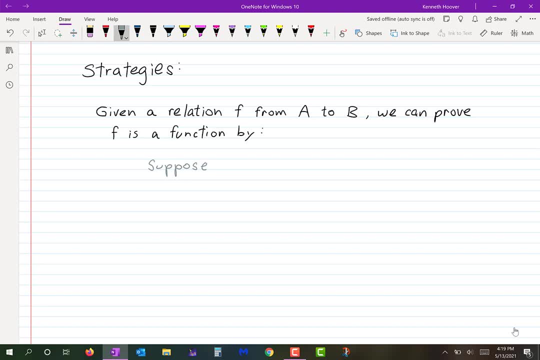 a, b is in f and a- let's say b prime is in f for some, a in the set a and b and b prime in the set b, and then you show that b must equal b prime. That's the standard way of proving that a relation is a function. 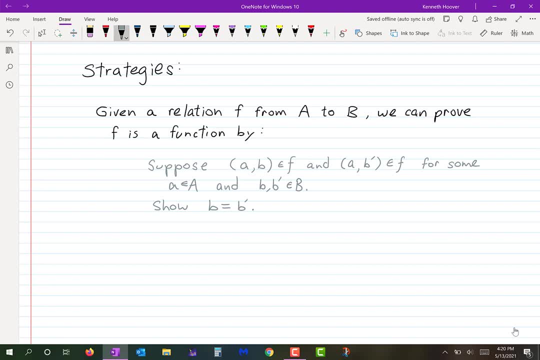 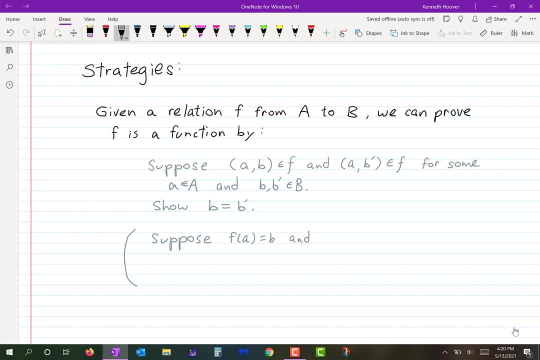 and f of a equals b prime for some a in a, for some a in a and b and b prime in b. show that b must equal b prime. show that b must equal b prime. show that b must equal b prime. 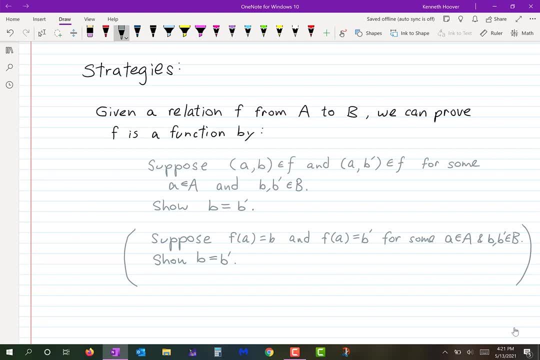 A lot of people do it that way, and that's actually the way I usually do it too. but I just will point out: hm, that is a little bit underhanded in a way, because we technically should not be writing this kind of a. 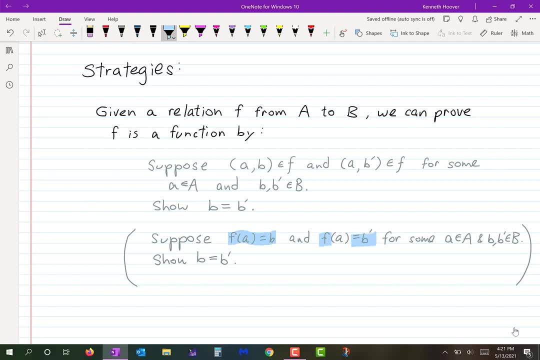 thing here: unless we know, f is a function, And so how can I be writing that when I'm trying to prove that f is a function? Because if I haven't proven it yet, then I wouldn't know that it's a function and so I wouldn't be writing it that way. 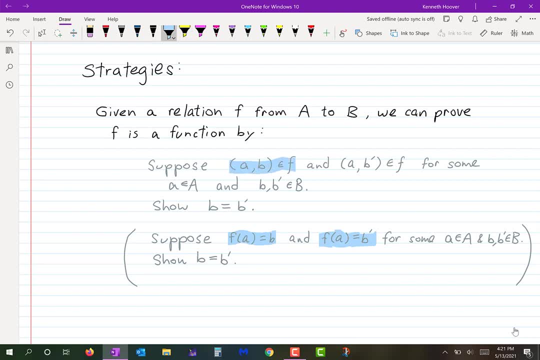 So technically, it should be written this way until you have proven it's a function. However, that's a technicality that most people overlook. Okay, now, that's how you prove a relation is a function. How do you prove that a function is? 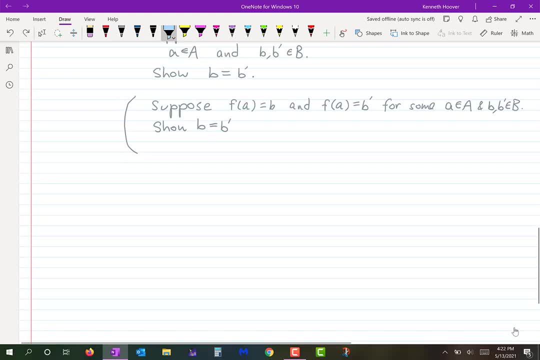 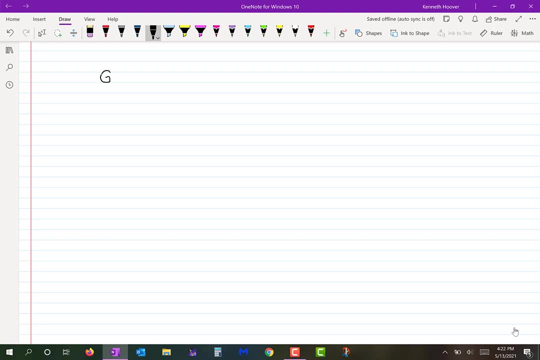 one to one. Okay, given a function f from a to b. Now, by my writing this, by my writing f, colon a, arrow b, that is indicating that I already know this is a function, I've already proven that or been told that, or whatever. Okay. 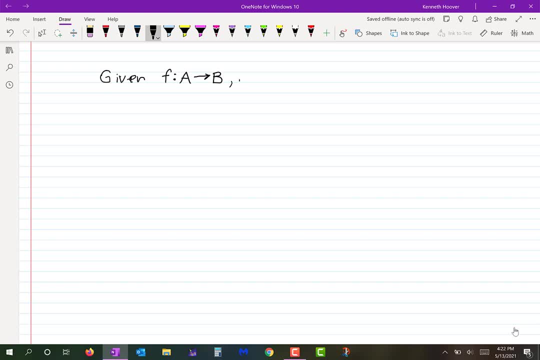 So, given a function from a to b, we prove: f is an injection by, f, is an injection by f, is an injection by a to b And it's an injection by an F of a and f of a prime equals b, F of a equals b. 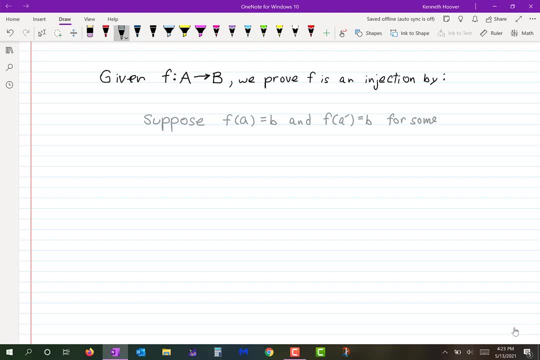 F of a equals b and f of a prime equals b. for some some B and B. and then you show that a must equal a prime. so that's saying that if one output comes from two inputs, then in fact of those inputs have to be the same, meaning that each output actually only comes from one input. so the 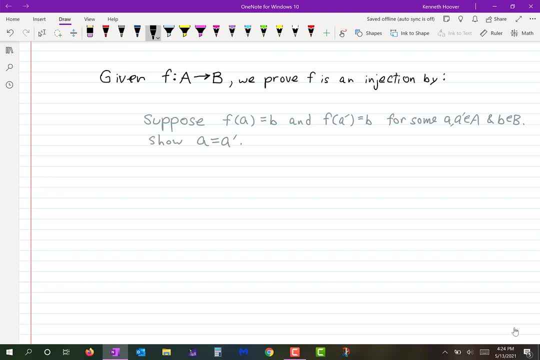 function is one-to-one okay. and finally, how do you prove surjectivity, given F from A to B, we prove F is a surjection by: suppose B is an element of the codomain. show B equals F of A for some A in the domain. ok, let's practice doing these kinds of proofs. 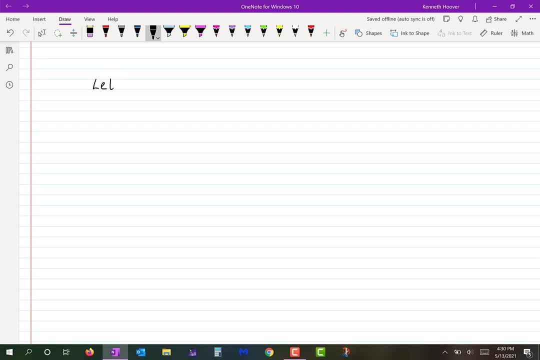 ok, let's write this one down. here is an example: let F be a function from the integers to the integers. ok, the FB whoops defined, ok, ok, ok, ok. Neutrality: A, B, B, D, E, A, A, W, D, E, T, W, B, B, K, K. 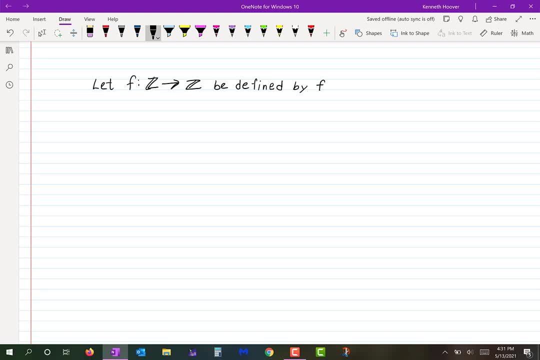 K by F of N. F of N. F of N equals two. n plus one equals two n plus one. F of N. okay, here's what we're going to do: verify that is in fact a function. prove that it's a bijection. okay, so now this is out of the book is number five and it. 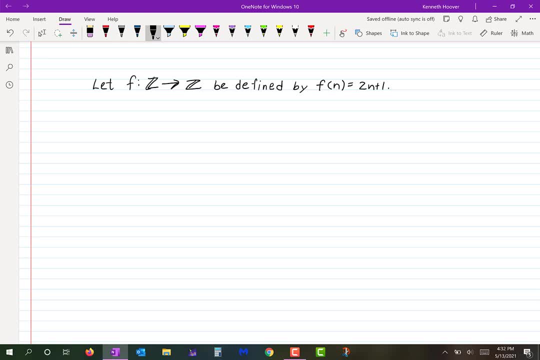 just says: verify whether it's injective or surjective. okay, so I'm actually adding to it. how would I show that this is a function? okay, so here's proof that F is a function. okay, and just follow that strategy that I set up above. okay, okay, so I'm going to show that this is a function. okay, so I'm going to show that. 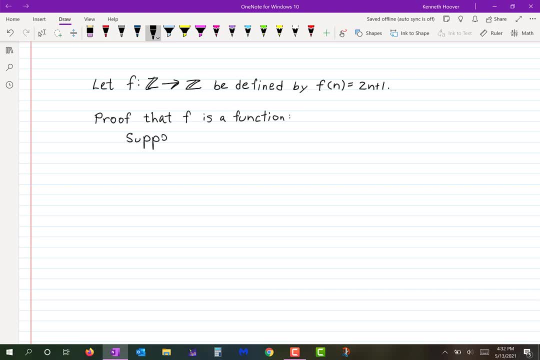 suppose there exists B and B prime. oh, since we've been given here that the codomain is the integers, then how about if we do this? how about if we say M and M prime? suppose there exists M and M prime in the integers, such that F of n equals M and f of n equals M prime. 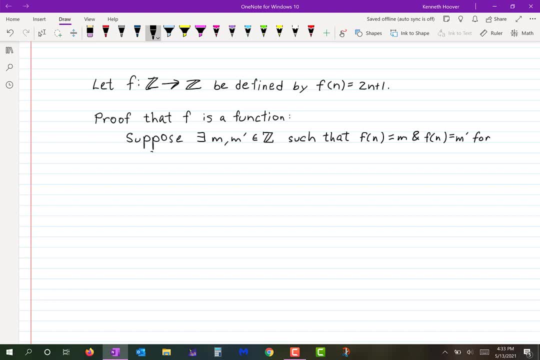 for sum n in the integers. this isn't going to be super easy. in fact, that's what confuses people a lot of the time. they feel like, well, there's nothing to do, so I don't know what to do. okay, but just bear with me here. then. M equals 2n. 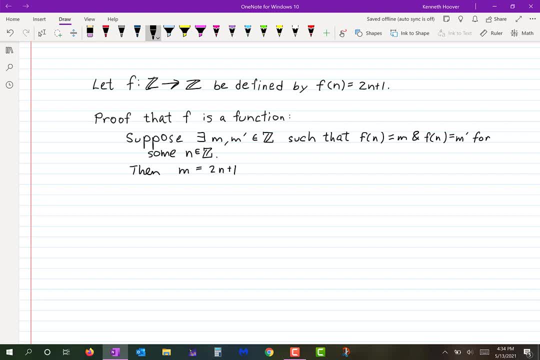 plus 1 and M, M, M, M M prime equals 2n plus 1. thus M equals M prime. so F is a function. okay now, believe it or not, we actually used some sophisticated stuff. do you remember talking about equivalence relations and the idea of equivalence relations and 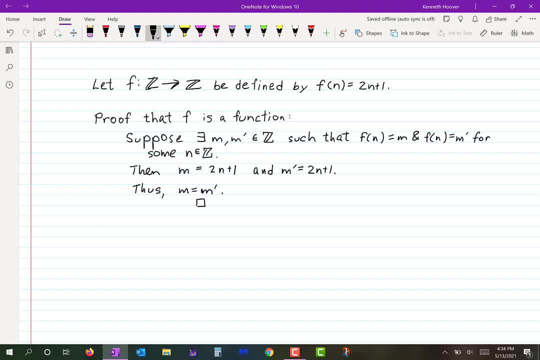 reflexivity, symmetry and transitivity. well, equality is an equivalence relation. in other words, equality is reflexive. every number is equal to itself. equality is symmetric: mm. we also have a pliable leverage number and the second number equals a third number and the first number equals a third number. we actually just used the symmetry and transitivity of equality. 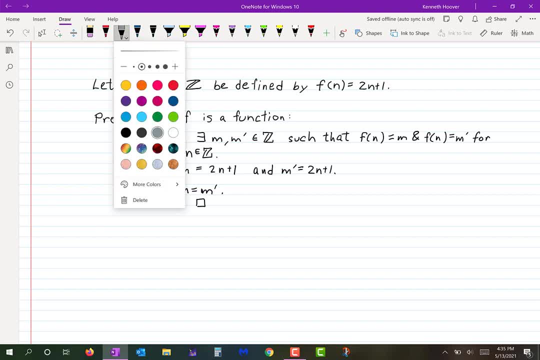 there, because what we did was we used the fact that M is 2n plus 1 and M prime equals 2n plus 1. we used symmetry to write: M equals 2n plus 1 and 2n plus 1 equals M prime. you see, I just used the symmetry right here, and then we use the. 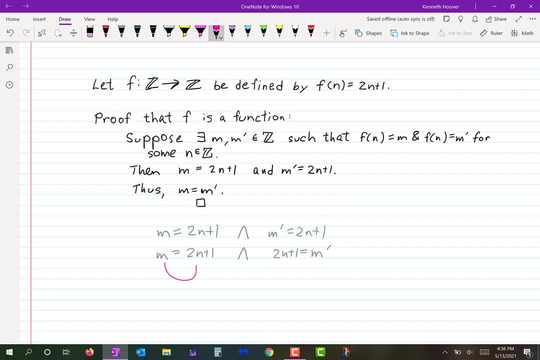 transitivity, because M equals this and that equals this, in fact. in fact, let's even write it this way: M equals 2n plus 1, and 2n plus 1 and 2n plus 1 equals M prime, and therefore M equals M prime. so 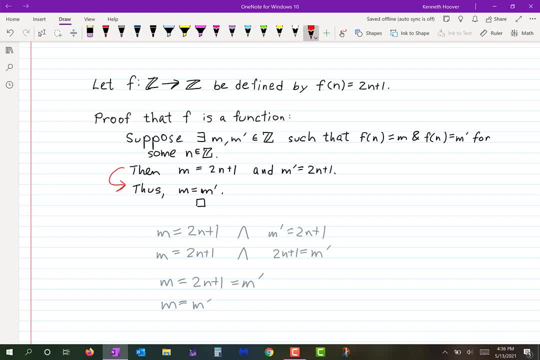 it seems like we didn't really do anything from here to here, but we actually did okay anyways. so we have verified that it is a function and, by the way, I allowed myself to write this notice. I did allow myself to do that and I felt justified in doing that, because they've already said this. 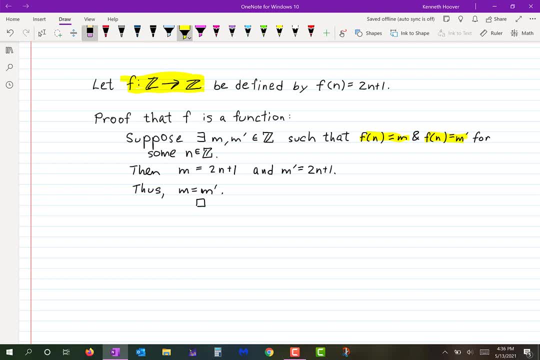 and I felt justified in doing that because they've already said this up here. they've already said that this is a function, and what I'm doing is I'm verifying that what they said is true. if they said: here's a relation, prove that it's a function, then I would try not to use that symbol over here until I had 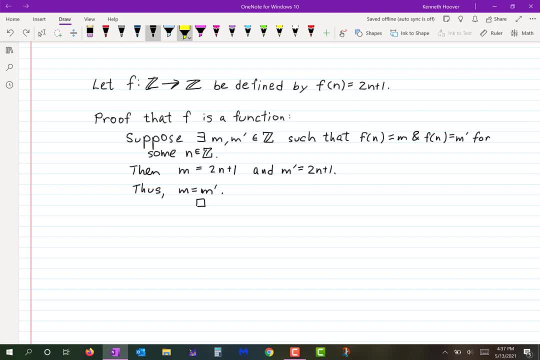 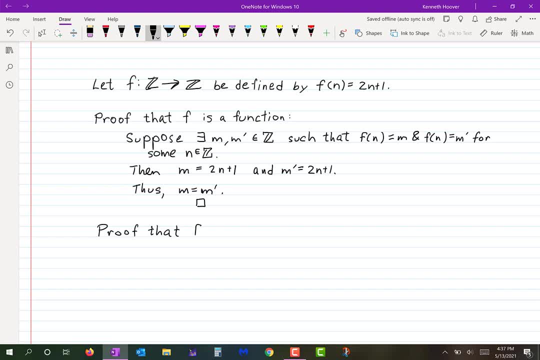 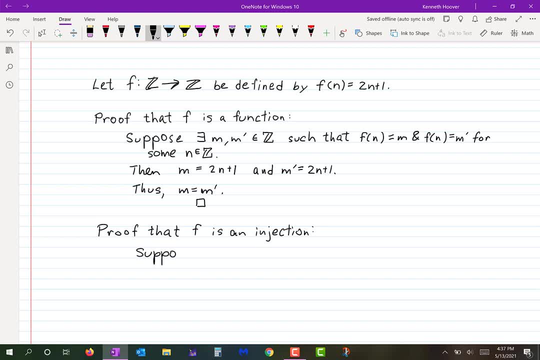 enough to make it interesting, okay enough to make it interesting, okay. so suppose there exists, there exists. there exists an n and an n prime in the integers, such an n and an n prime in the integers, such an n and an n prime in the integers, such that f of n equals m and also f of n. 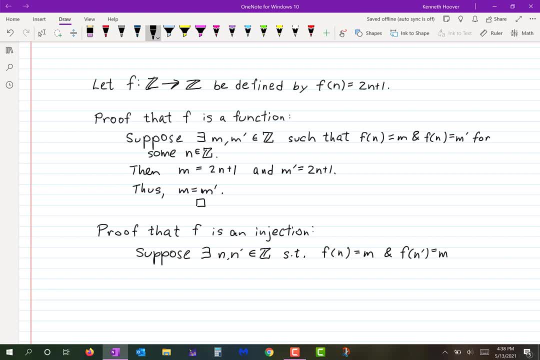 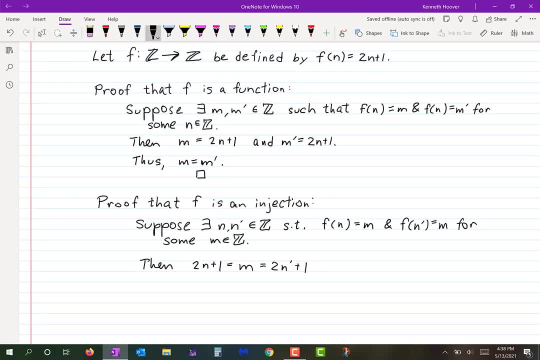 we're just going to write it as one string of. we're just going to write it as one string of. we're just going to write it as one string of Equality. okay, Hence, 2n plus 1 equals 2n prime plus 1.. 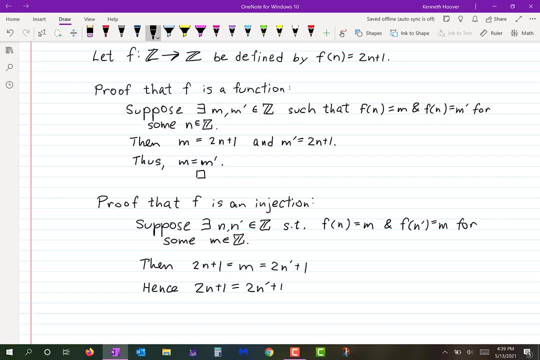 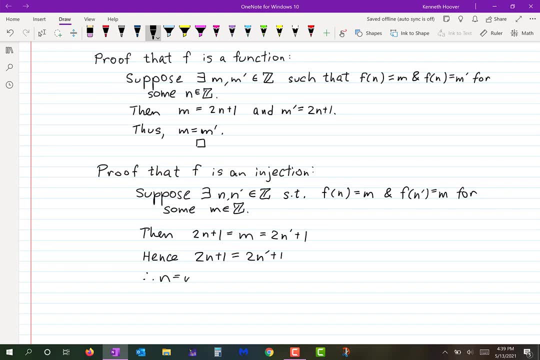 And we're just going to do some algebra here, Because this is specifically. I want to do this for practice, so I'm not going to just jump to the end and say, therefore, n equals n prime. No, let's actually. let's write down how you would get there. 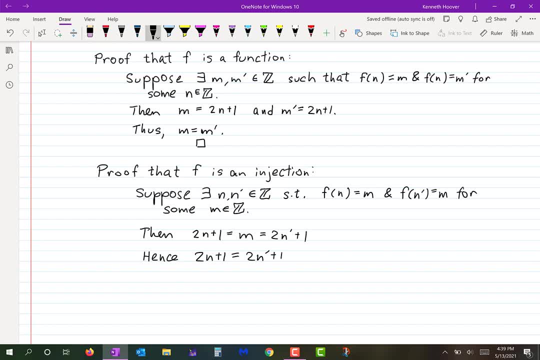 Okay, I'm not usually this specific, but I'm actually going to write down by sorry. I said adding. I should have said subtracting. by subtracting 1 from both sides, We get 2n equals 2n prime. 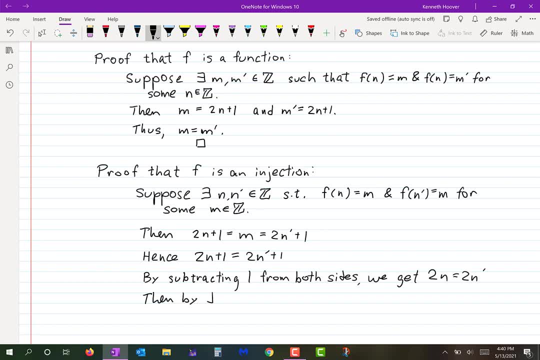 Then, by dividing both sides by 2, we have n equals n prime, And there we go, Okay, Okay, So it is in fact an injection, isn't it Okay? How would you prove it is a surjection? 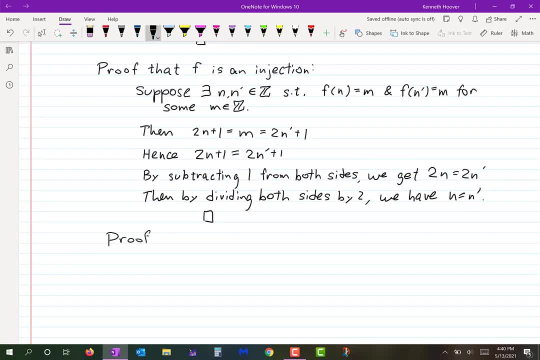 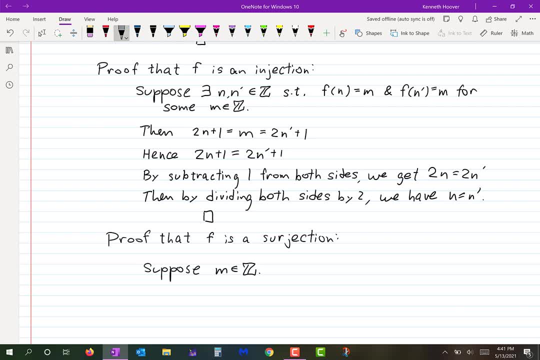 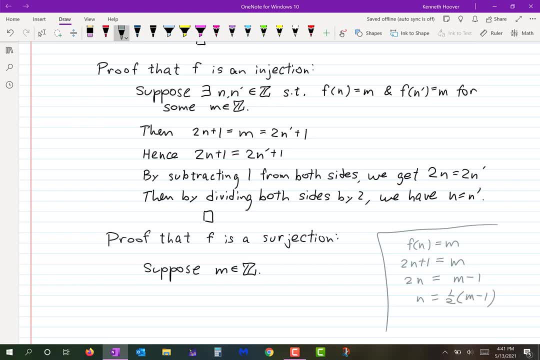 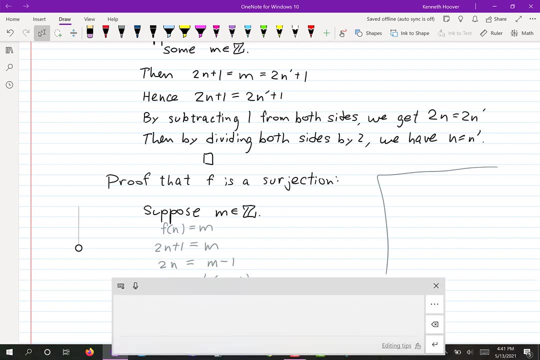 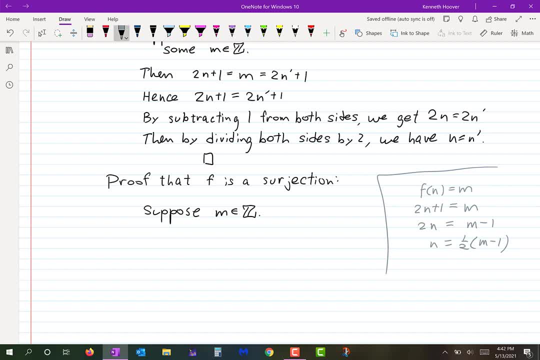 Scratch work is what you do to figure out the proof. I need to figure out something in the integers that is going to get mapped to m And I did the scratch work to figure that out. Now what I do is I need to show actually two things. 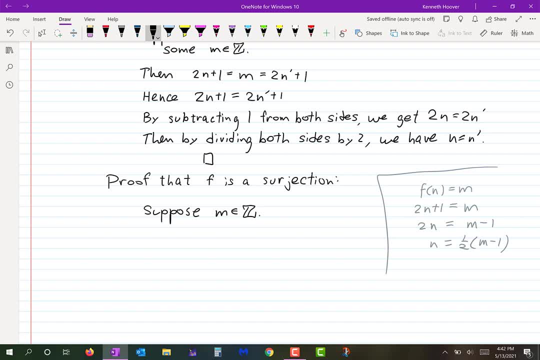 I need to show that the thing I found is in fact in the domain of f, And then I need to show that the thing that I found will get mapped to m. So back to our proof. Suppose m is an integer, Then one half m minus one is an integer, Correct. 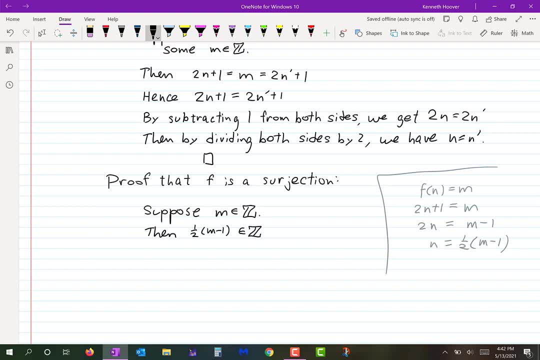 Yes, that is correct, because subtracting from m is an integer. So subtracting one from an integer and then dividing it by two will still give you an integer. Also, f of one half m minus one would equal what would it equal? It equals two times one half of m minus one plus one. 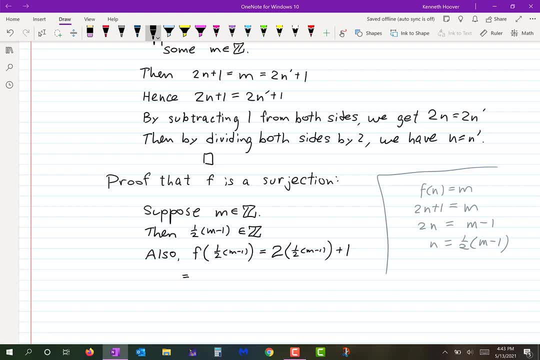 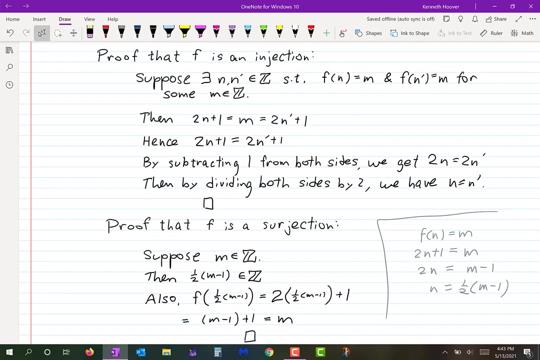 Which equals m, minus one plus one which equals m. So I found something that gets mapped to m. I showed that that thing is in the domain and it gets mapped to m, And so that means that f is surjective. That's a strategy of how you prove injectivity and surjectivity. 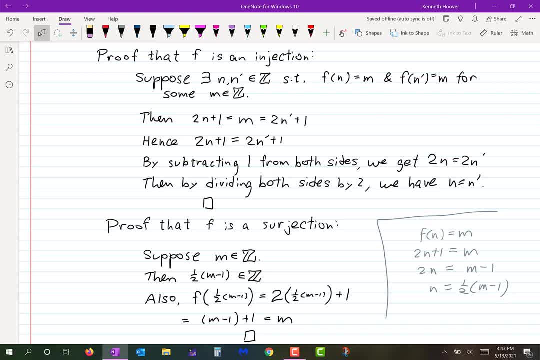 Okay. They are important concepts. Knowing how to prove them is important. As I was writing this, it dawned on me to maybe point out one other thing Up here for injectivity. I started off by saying: suppose there exists n and n prime such that f of n equals m and f of n prime equals m, for some m in the integers. 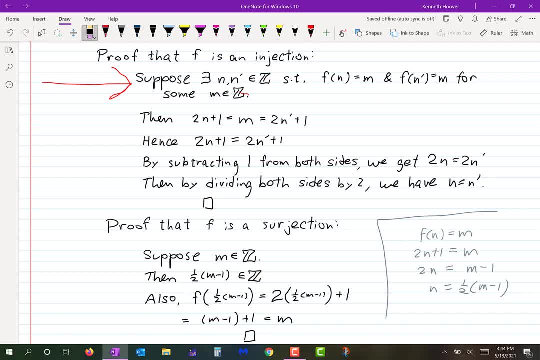 It dawned on me that there is a slightly shortened way that people often write that which is totally acceptable. So let me just show you real quick. It actually saves some space And this is totally fine to do. You can say: suppose there exists an n and n prime in the integers, such that f of n equals f of n prime. 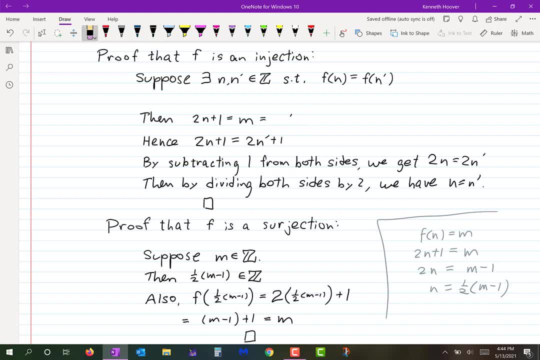 In that case, there is no mention. There is no mention of any m. So then, in that case you can go straight to. well, my computer is not cooperating, so let me just tell you that you can just bump this up, then That's actually a good way to do the proof. 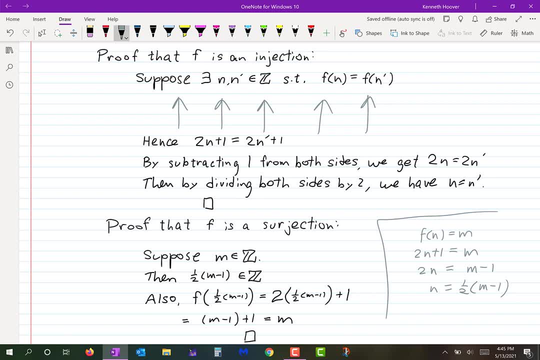 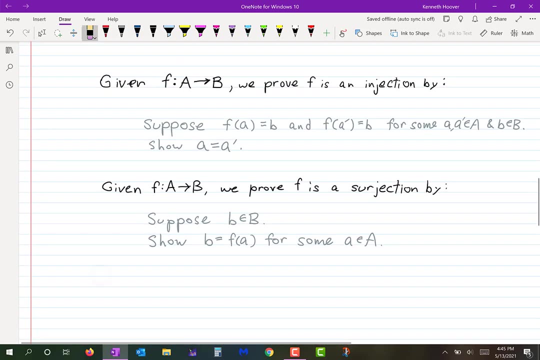 It eliminates that third variable. m Also eliminates what was the second line. Okay, So maybe you should do them that way, It's better. Let me look back at what I wrote up here for my strategy for injection. See where I wrote: suppose f of a equals b and f of a prime equals b. 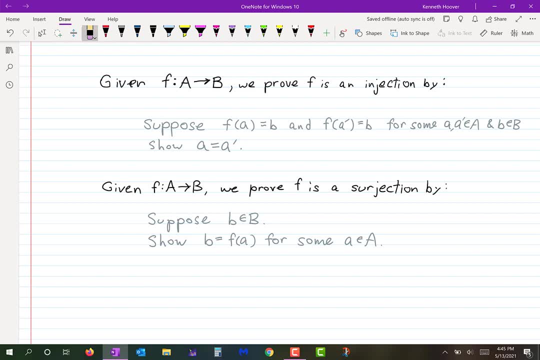 So for some a and a prime and some b. So maybe it's better then if we reword that in this more efficient way And say: Suppose f of a equals f of a prime for some a and a prime in the domain. That's more efficient that way. Okay, Alright, That's it for today.